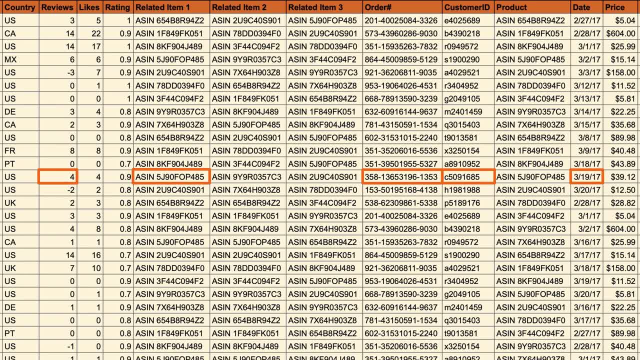 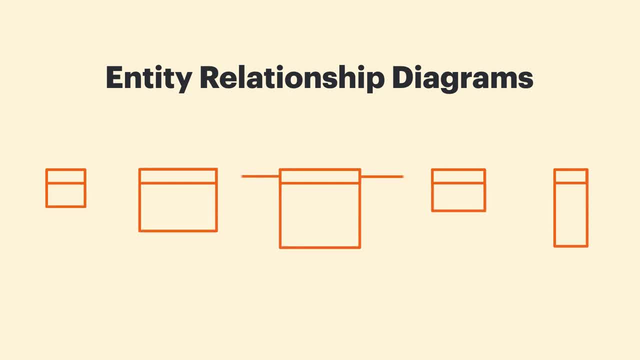 in a database, and understanding how each of these elements interacts with one another can be a very important part of a database. ERDs provide engineers with a visual way to understand how this information is related and how it works together. So how do we make one? Today, I'm going to be using Lucidchart. 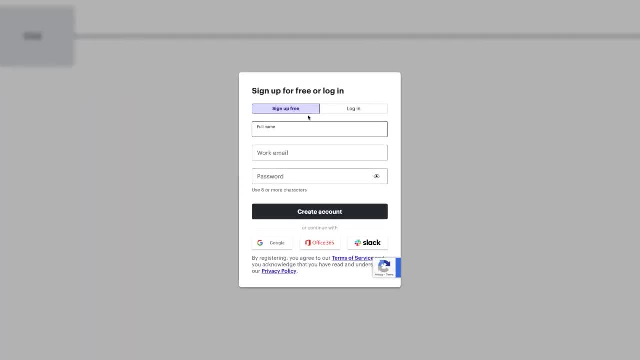 and you can too, for free, actually, By clicking on the top right corner, you can access Lucidchart's website into your email address and have a free account in just a few seconds. That way, you can follow along with me and create your own ERDs in the future. Okay, 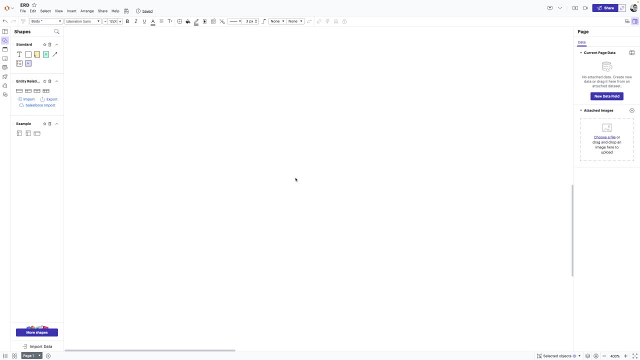 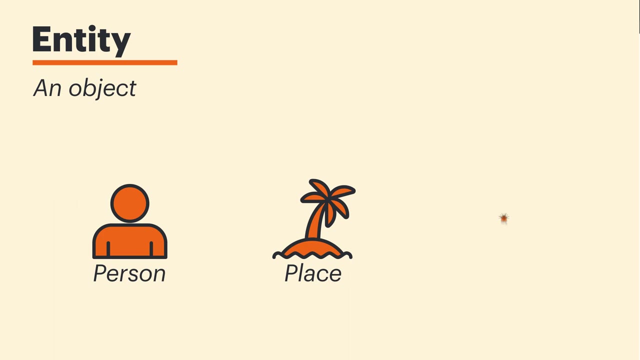 so, in order to build an ERD, we need to better understand its individual components, And this starts with entities. An entity is an object like a person, place or thing that's tracked in the database. For example, if we were to buy something on Amazon, say. 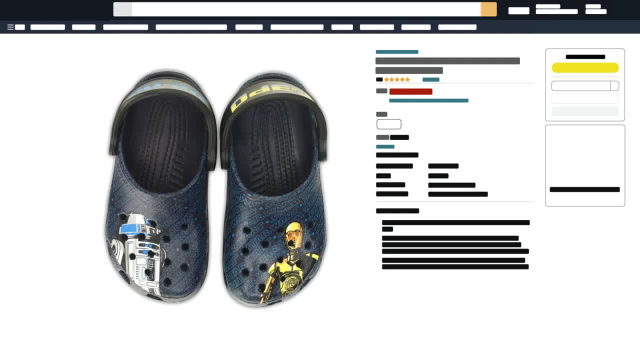 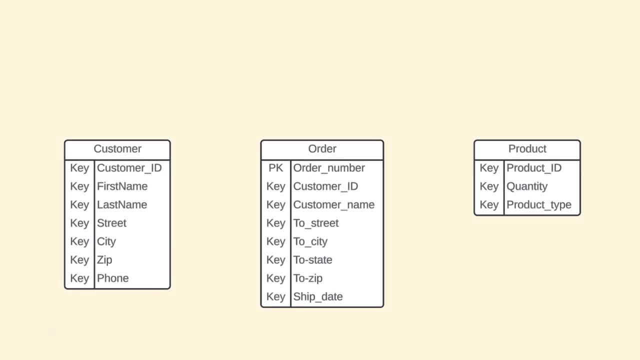 a rockin' pair of Crocs. an entity could be the customer, the order and, of course, our Crocs, the product. Now, each of these entities will have attributes, which are properties or traits, In this case under the customer entity. 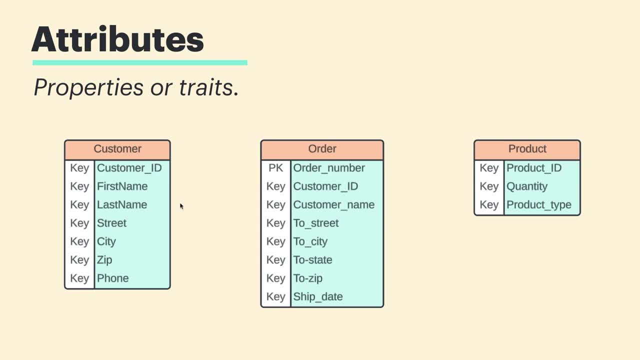 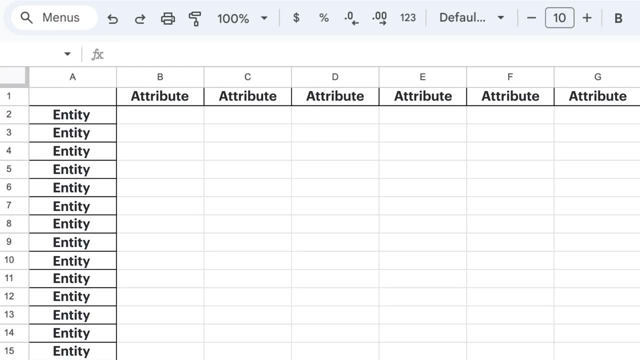 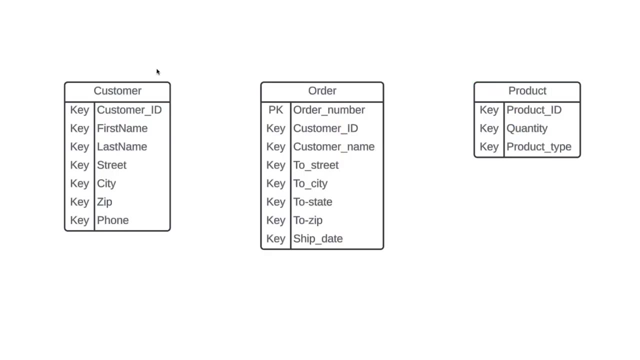 we have customer ID, first name, last name, street, city, zip and phone. It's important to note that entities in your database will always be depicted as rows and that attributes will always be depicted as columns, And now that we have these different. 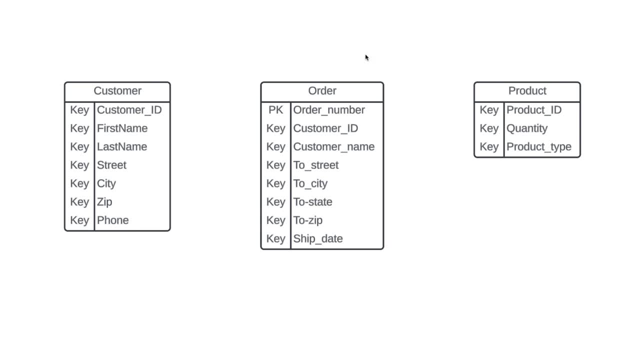 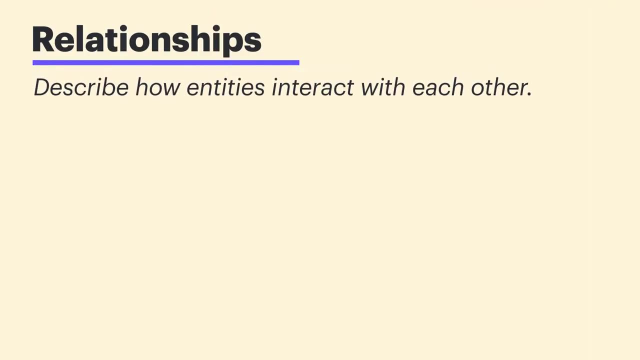 entities and attributes on the screen. here we can talk about the relationships that exist between them. Relationships describe how these entities will interact with each other. So when I draw a line between these particular elements, I'm showing that there's some sort of 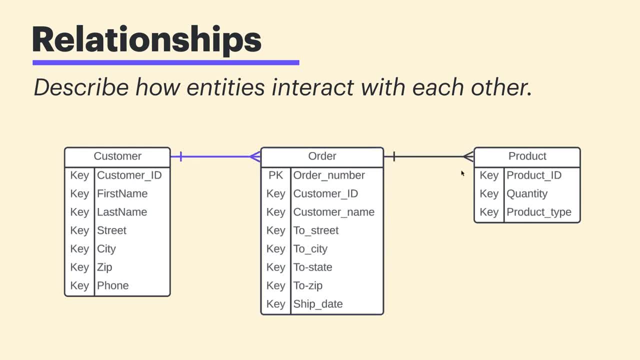 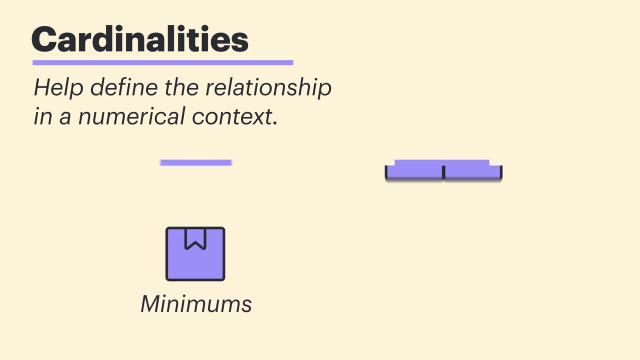 connection. And now that we have our relationships in place, we'll see an interesting notation attached to our lines. This is called cardinality. Cardinalities help define the relationship in a numerical context, particularly within minimums and maximums, For example. 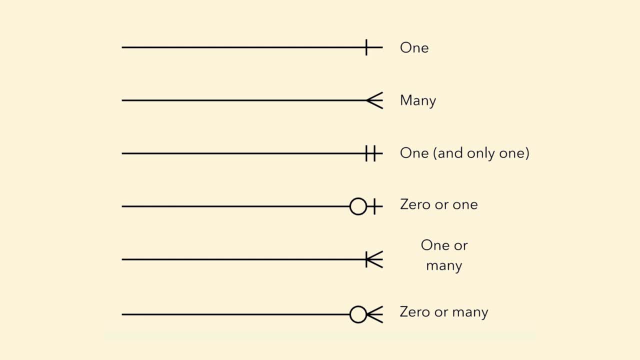 this list shows some of the different cardinalities that can appear in an ERD. We have one many, one and only one zero, or one one or many and zero or many. And if this isn't making sense yet, don't worry, We'll walk through a few examples to help piece. 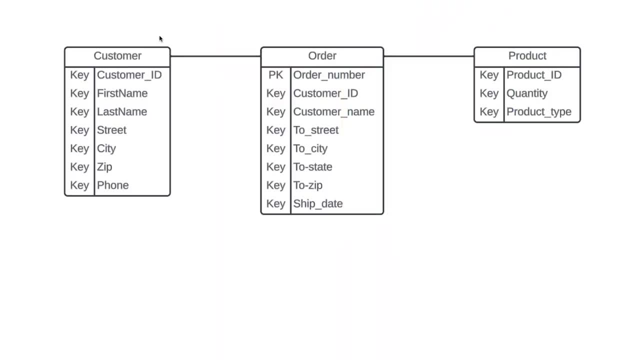 everything together. Let's start by talking about the relationship and cardinality that exists between customer and order. The best way to do this is to think about it logically, So we should ask ourselves two questions: What is the minimum number of orders that a customer 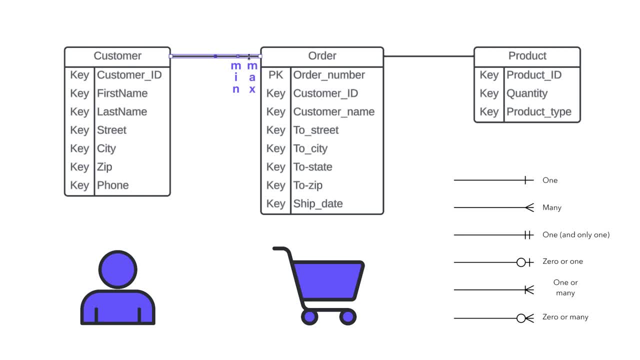 could have. And two, what is the maximum number of orders that a customer could have? Well, a customer could exist, but he or she could have zero orders. So to show that we'll have that zero sign, Now we need to think about the maximum And, as you've probably assumed, 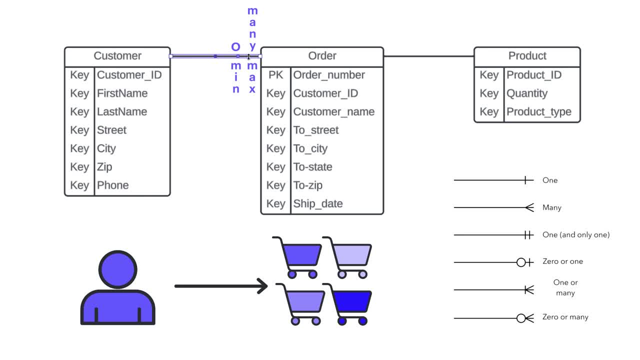 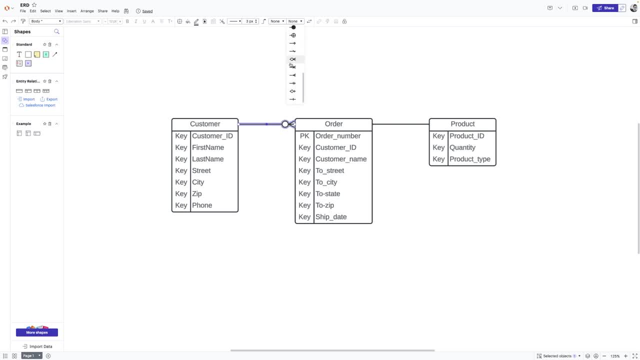 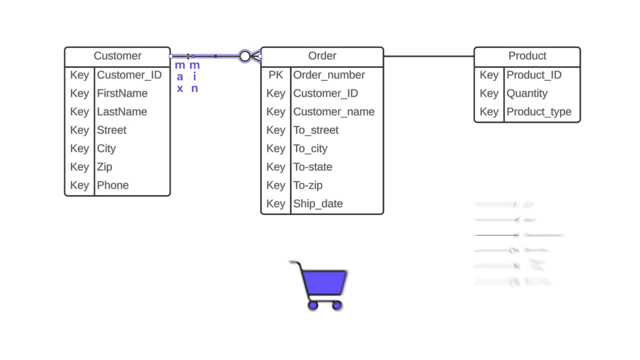 a customer could have an infinite number of orders. especially when it comes to Crocs, You can never have just one. So to show that we'll use this zero or many crow's foot notation, Now let's talk about the minimum and maximum relationship between orders and customers. 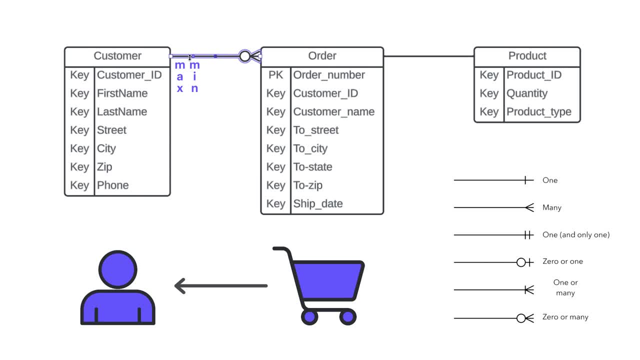 We'll start by applying the same logic. So we'll ask ourselves: what is the minimum amount of customers that an order may have, And what's the maximum amount of customers that an order may have? A specific order can have one and only one customer. Imagine the confusion that would. 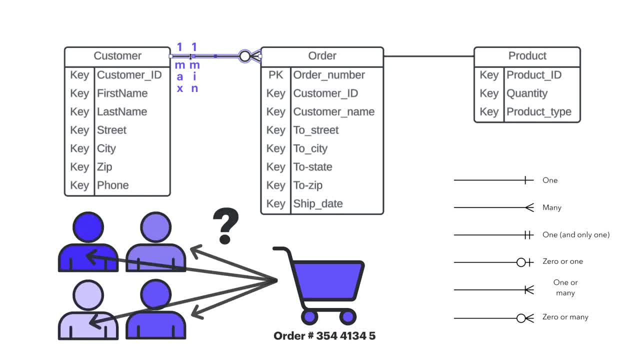 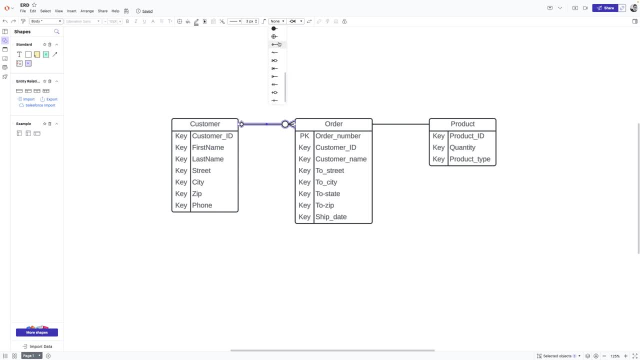 come if the same specific order had a lot of customers. So in this case there can be one and only one number of customers to order, And we show that using this sign here. Now let's talk about the relationship or cardinality between orders and products. 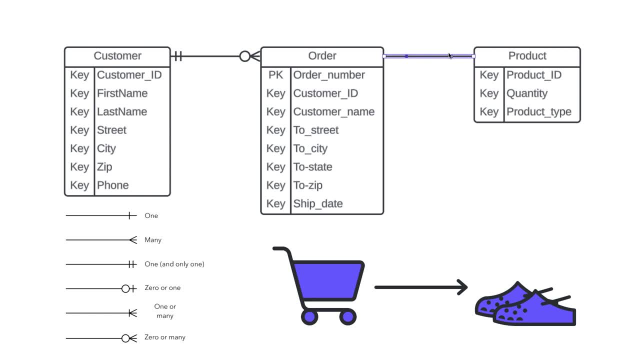 We'll ask ourselves a similar question: A certain order can have how many products? Well, for an order to exist, it has to have one product, But a lot of different products can be part of that order. So let's say that an order can have one and only one customer, And we'll ask: 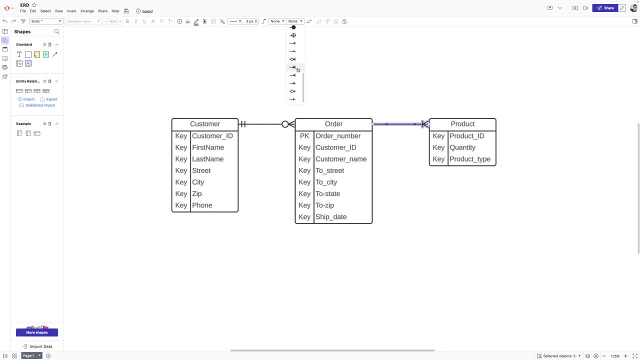 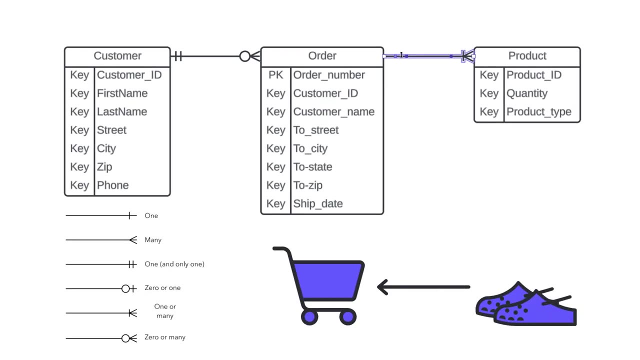 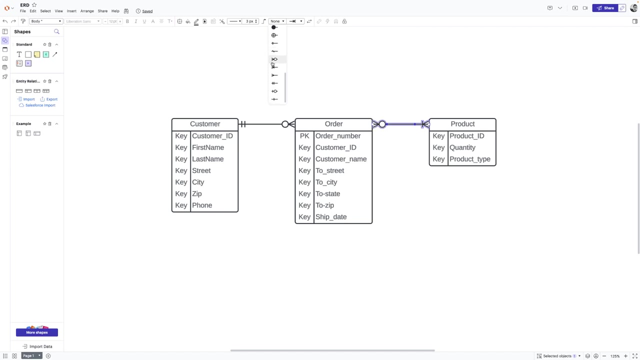 ourselves that question in reverse: A product can be a part of how many orders? Well, a product could be a part of no orders, but it could also be a product of many orders. So we're going to use this zero or many notation on our diagram And just like that we've built an entire entity. 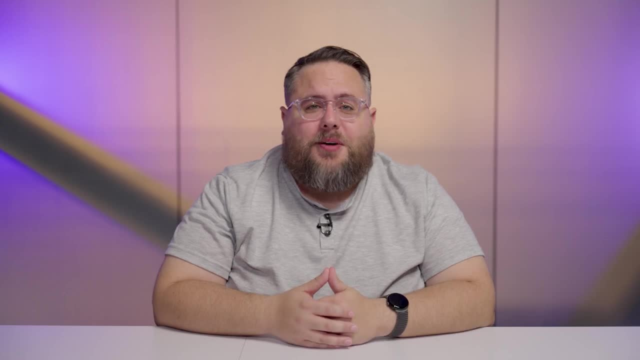 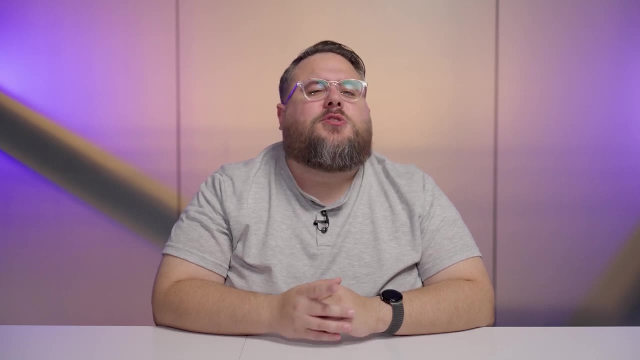 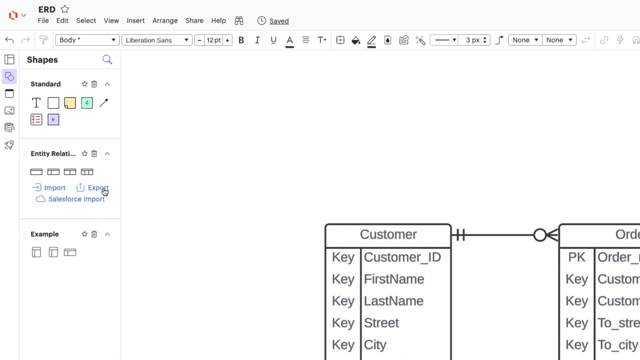 relationship diagram, And even though it's a simple example, you should now have the basic skills needed to build a complex one. And not only that, but because you used Lucidchart, you also have the option to export this diagram directly into a database Using the export feature.